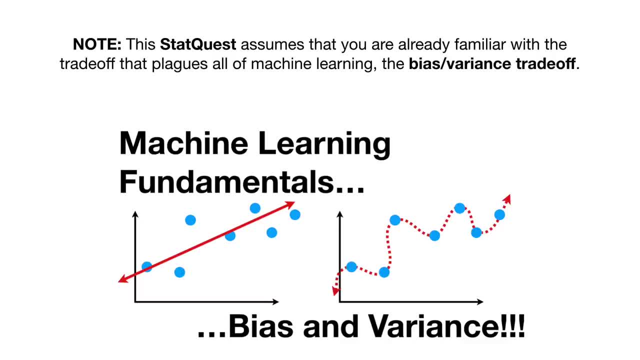 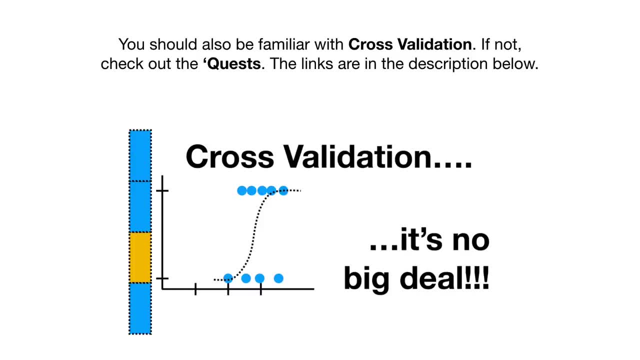 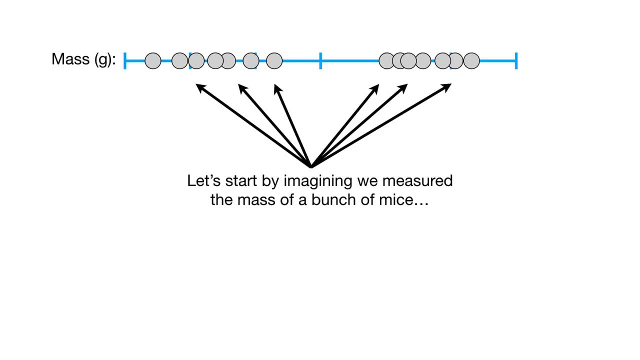 that you are already familiar with the trade-off that plagues all of machine learning, The bias variance trade-off. You should also be familiar with cross-validation. If not, check out the quests. The links are in the description below. Let's start by imagining we measured the mass of a bunch of mice. The red dots represent mice. 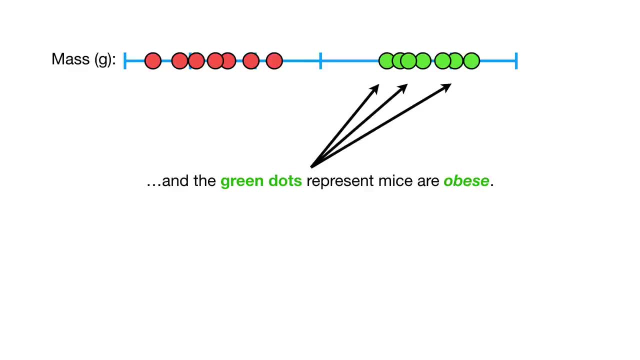 that are not obese and the green dots represent mice that are obese. Based on these observations, we can pick a threshold, and when we get a new observation that has less mass than the threshold, we can classify it as not obese, And when we get a new observation with more mass than the threshold, we can classify it. 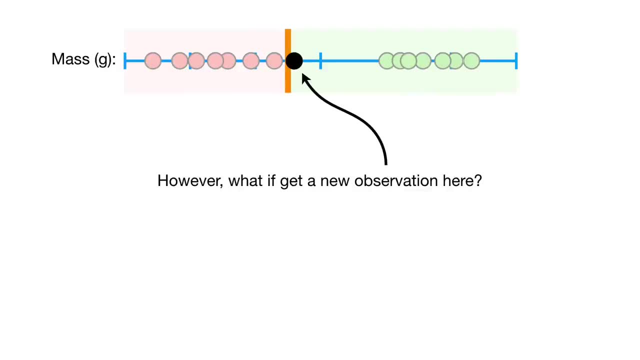 as obese. However, what if we get a new observation here? Because this observation has more mass than the threshold, we classify it as obese. But does that mean this observation is tune and game over? não é cada vez mais obscura que o threshold, e quando chegamos à nova observação com mais massa do que o threshold, podemos classificá-lo como obesso? 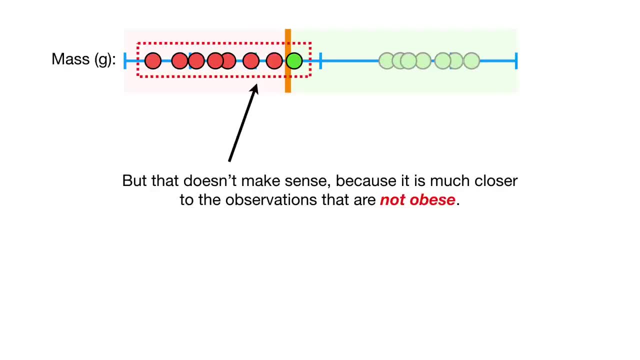 that doesn't make sense because it is much closer to the observations that are not OBs, So this threshold is pretty lame. Can we do better? Yes, Going back to the original training data set, we can focus on the observations on the edges of each. 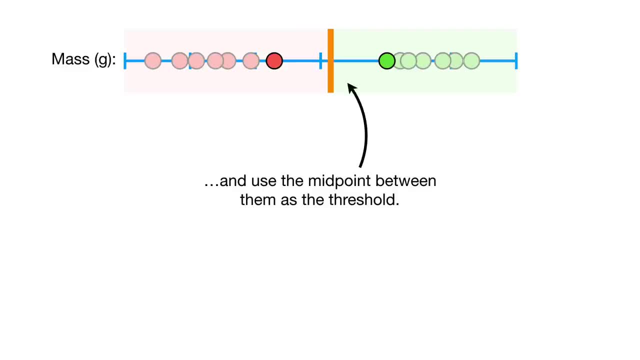 cluster and use the midpoint between them as the threshold. Now, when a new observation falls on the left side of the threshold, it will be closer to the observations that are not OBs than it is to the OBs observations. So it makes sense to classify this new observation as not OBs. BAM. 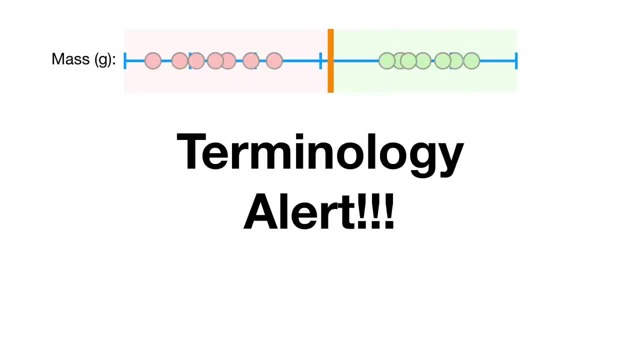 Oh no, It's a terminology alert. The shortest distance between the observations and the threshold is 0.5.. The threshold is called the margin. Since we put the threshold halfway between these two observations, the distances between the observations and the threshold are the same. 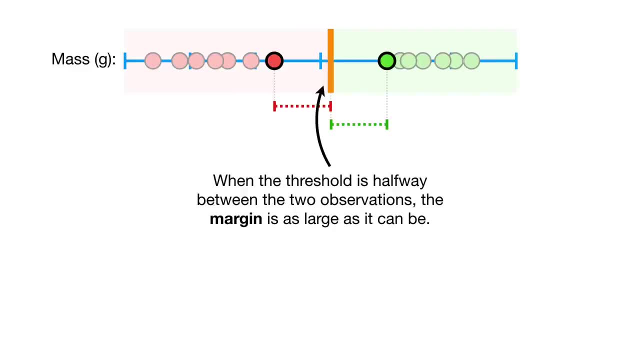 and both reflect the margin. When the threshold is halfway between the two observations, the margin is as large as it can be. For example, if we move the threshold to the left a little bit, then the distance between the threshold and the observation that is not obese would be smaller, and thus 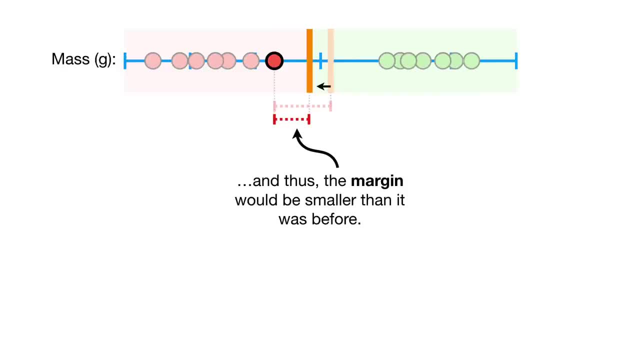 the margin would be smaller than it was before. And if we move the threshold to the right a little bit then the distance between the obese observation and the threshold would get smaller and again the margin would be smaller. When we use the threshold, that gives us the largest margin to make classifications heads. 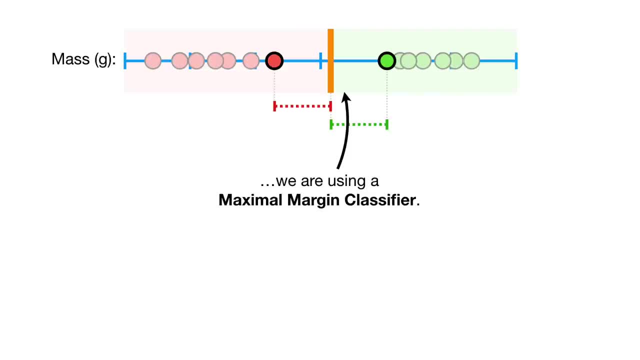 up terminology. alert: we are using a maximal margin classifier. Bam, No, No, bam. Maximal margin classifiers seem pretty cool, but what if our training data looked like this And we had an outlier observation that was classified as non-existent? 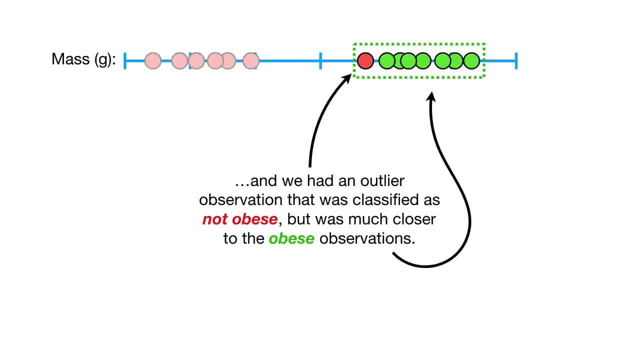 It was not obese but was much closer to the obese observations. In this case, the maximal margin classifier would be super close to the obese observations and really far from the majority of the observations that are not obese. Now, if we got this new observation, we would classify it as not obese, even though most 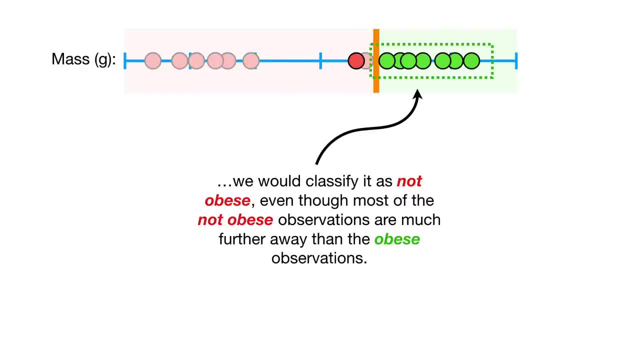 of the not obese observations are much further away. So maximal margin classifiers are super sensitive to outliers in the training data and that makes them pretty lame. Can we do better? Yes, To make a threshold that is not so sensitive to outliers. we must allow misclassifications. 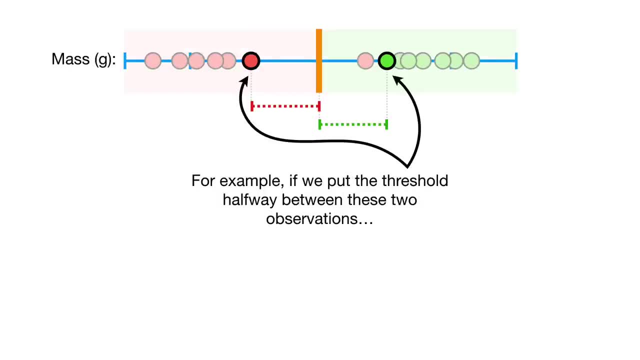 For example, if we put the threshold halfway between these two observations… Then… Then we will misclassify this observation. However, now when we get a new observation here… We will classify it as obese, And that makes sense because it is closer to most of the obese observations. 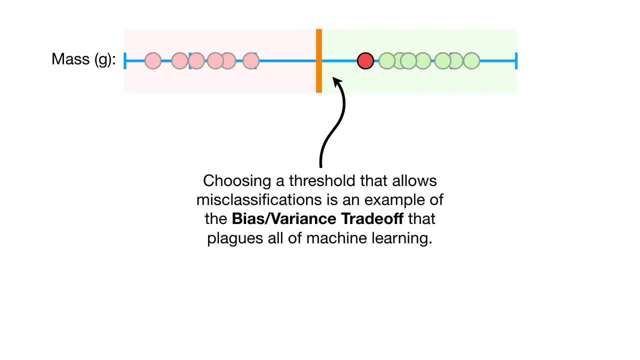 Choosing a threshold that allows misclassifications is an example of the bias-variance trade-off that plagues all of machine learning. In other words… Before we allowed misclassifications, we picked a threshold that was very sensitive to the training data. It had low bias. 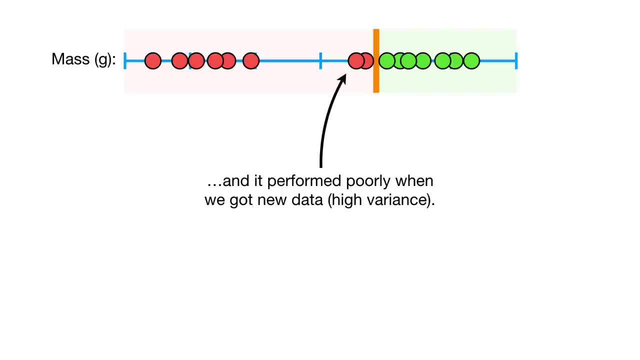 And it performed poorly when we got new data. It had high variance. In contrast, when we picked a threshold that was less sensitive to the training data and allowed misclassifications, so it had higher bias… It performed better when we got new data. 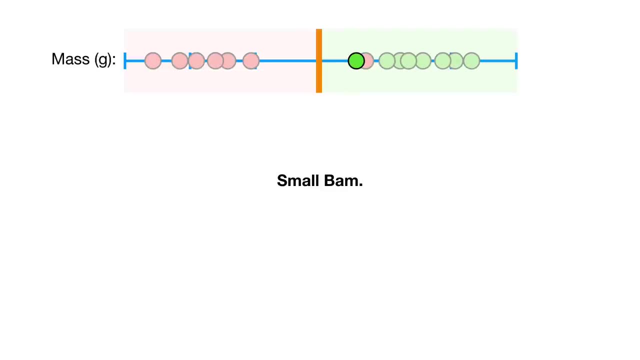 So it had low variance. Small bam, Oh no, It's another terminology- alert When we allow misclassifications. the distance between the observations and the threshold is called a soft margin. So the question is… How do we know that this soft margin…? 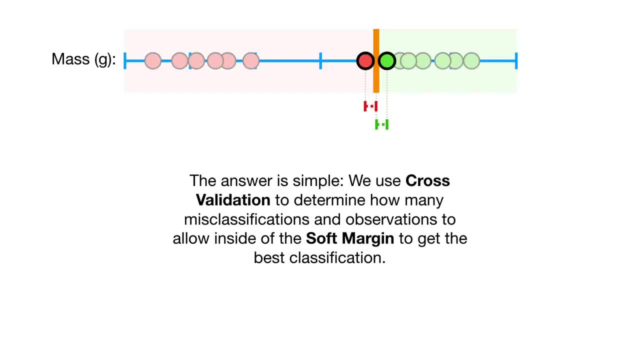 Is better than this soft margin? The answer is simple. We use cross-validation to determine how much margin is better than this margin, determine how many misclassifications and observations to allow, inside of the soft margin, to get the best classification. For example, if cross. 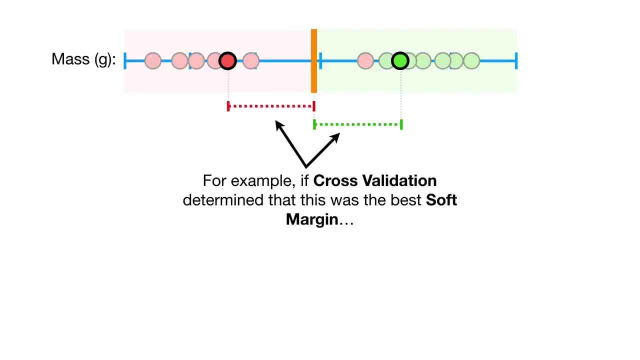 validation determined that this was the best soft margin, then we would allow one misclassification and two observations that are correctly classified to be within the soft margin. Bam, When we use a soft margin to determine the location of a threshold, brace yourself. we have another terminology. 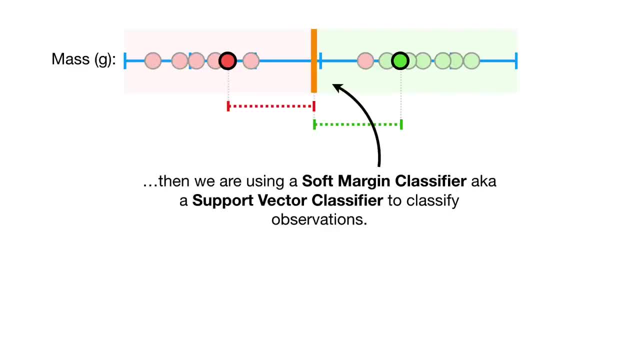 alert, then we are using a soft margin classifier, aka a support vector classifier, to classify observations. The name support vector classifier comes from the fact that the observations on the edge of the edge are then classified as observations and within the soft margin are called support vectors. Super small BAM. Note if 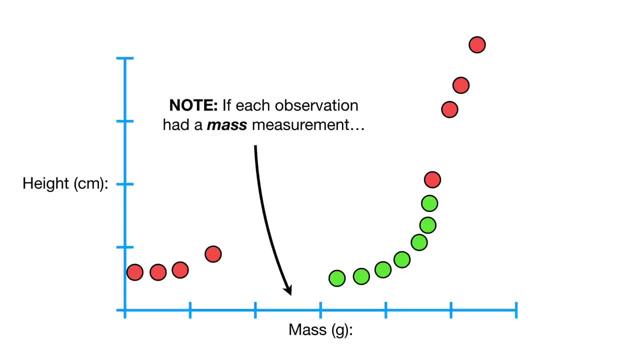 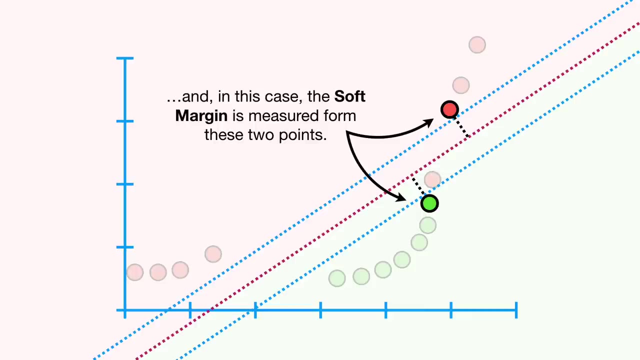 each observation had a mass measurement and a height measurement, then the data would be two-dimensional. When the data are two-dimensional, a support vector classifier is a line and in this case the soft margin is measured from these two points. The blue parallel lines give us a sense of where all of the other 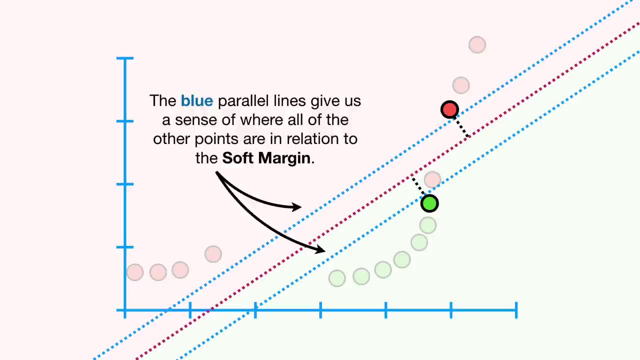 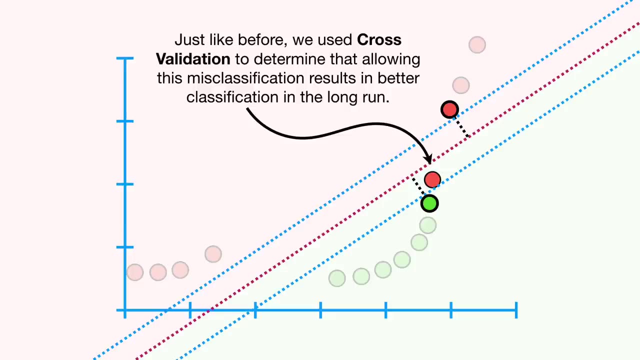 points are in relation to the soft margin. These observations are outside of the soft margin and this observation is inside the soft margin and misclassified, Just like before. we used cross validation to determine that allowing this misclassification results in better classification in the long run. BAM. 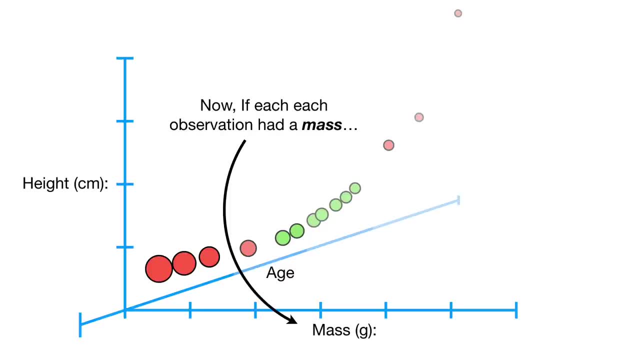 Now, if each observation has a mass, a height and an age, then the data would be three-dimensional. Note: the axis that age is on is supposed to represent depth, And, And these circles are larger in order to appear closer and thus younger. 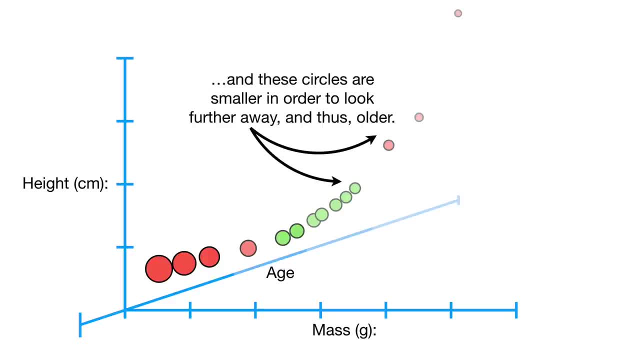 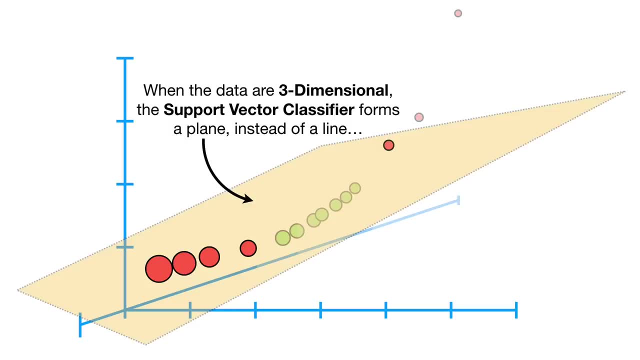 And these circles are smaller in order to look further away, and thus older. When the data are three-dimensional, the support vector classifier forms a plane instead of a line, And we classify new observations by determining which side of the plane they are on. For example, if this were a new observation, we would classify it as not obese, since it is above the support vector classifier. 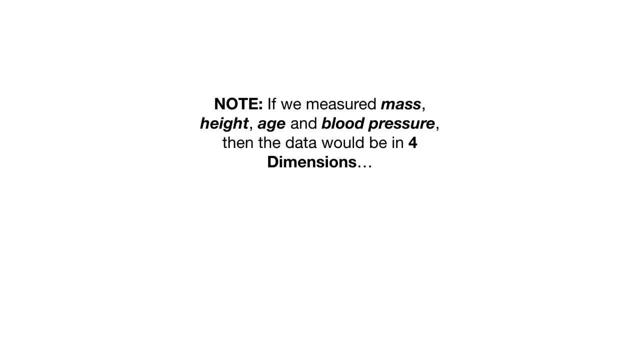 Note: if we measured mass, height, age and blood pressure, then the data would be in four dimensions, And I don't know how to draw a four-dimensional graph, Wah wah. But we know that when the data are three-dimensional, they are not obese. 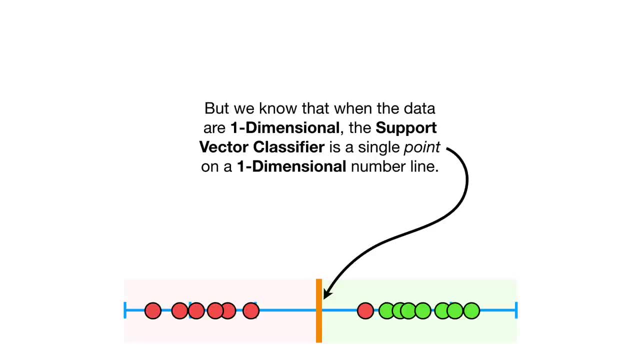 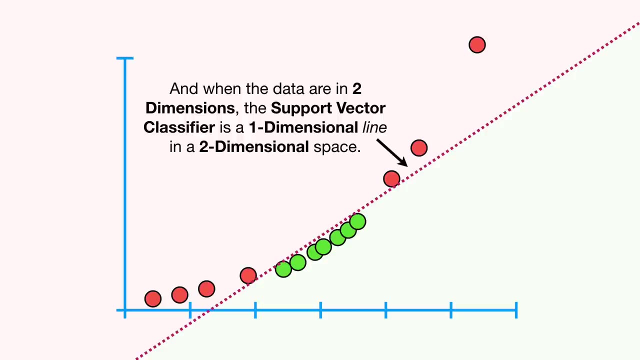 When the data are one-dimensional, the support vector classifier is a single point on a one-dimensional number line, Psst in mathematical jargon, a point is a flat, affine, zero-dimensional subspace. And when the data are in two dimensions, the support vector classifier is a one-dimensional line in a two-dimensional space. 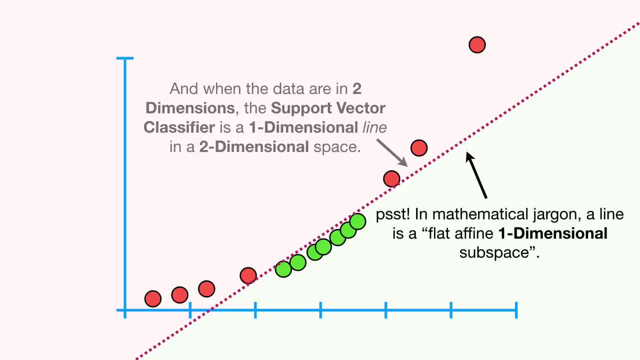 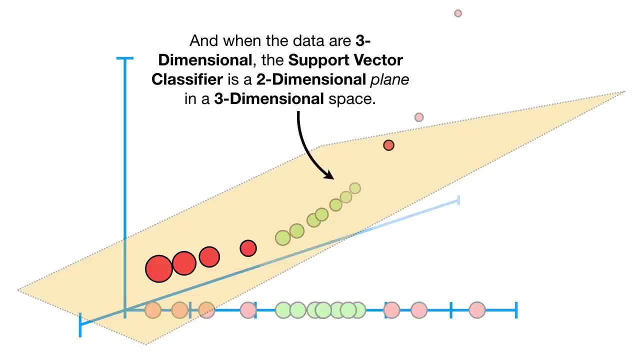 Psst. in mathematical jargon, a line is a flat affine one-dimensional space- Psst. in mathematical jargon, a plane is a flat affine two-dimensional subspace And when the data are three-dimensional, the support vector classifier is a two-dimensional plane in a three-dimensional space. 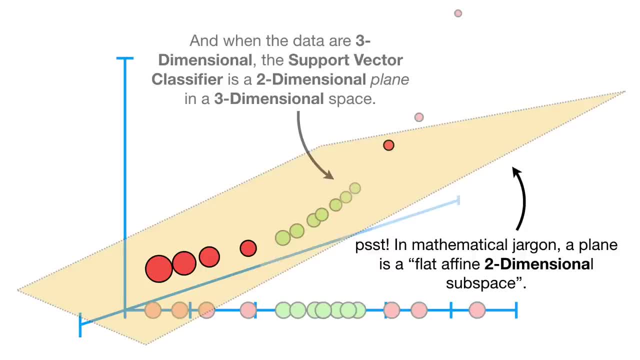 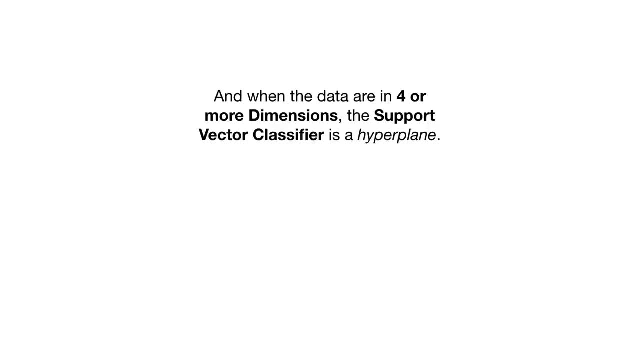 Psst. in mathematical jargon, a plane is a flat, affine, two-dimensional subspace, And when the data are in four or more dimensions, the support vector classifier is a hyperplane. Psst in mathematical jargon, a plane is a flat, affine, two-dimensional subspace. 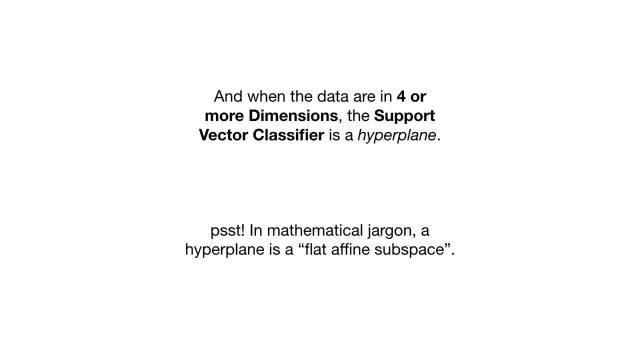 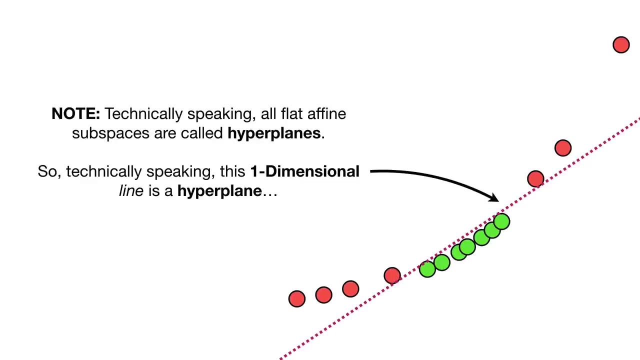 In mathematical jargon, a hyperplane is a flat affine subspace. Note: technically speaking, all flat affine subspaces are called hyperplanes. So technically speaking, this one-dimensional line is a hyperplane, But we generally only use the term when we can't draw it on paper. 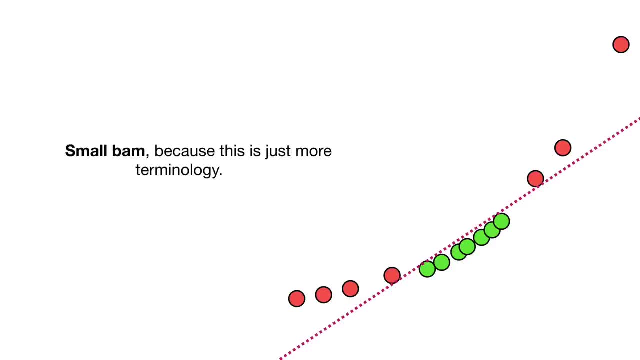 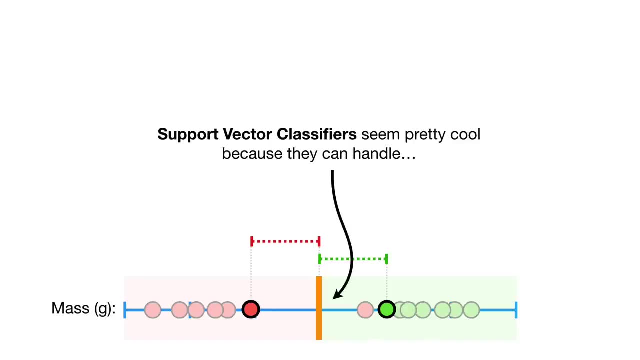 Small bam, because this is just more terminology. Ugg Support vector classifiers seem pretty cool because they can handle outliers And because they can allow misclassifications. they can handle overlapping classifications. But what if this was our training data and we had tons of overlap? 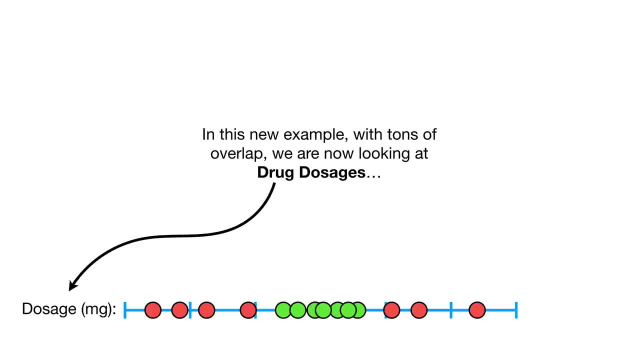 In this new example, with tons of overlap, we are now looking at drug dosages, And the red dots represent pathogens And the blue dots represent patients that were not cured And the green dots represent patients that were cured. In other words, the drug doesn't work if the dosage is too small or too large. 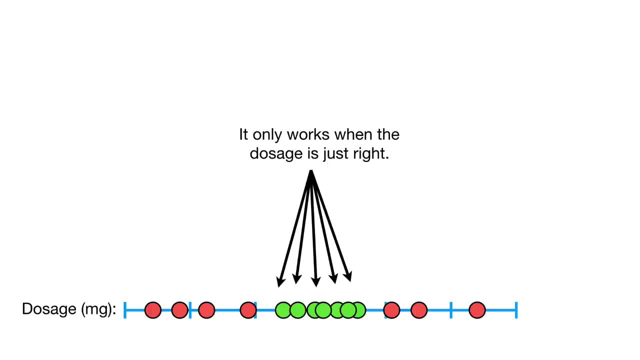 It only works when the dosage is just right. Now, no matter where we put the classifier, we will make a lot of misclassifications. So support vector classifiers are only semi-quick. So support vector classifiers are only semi-quick. 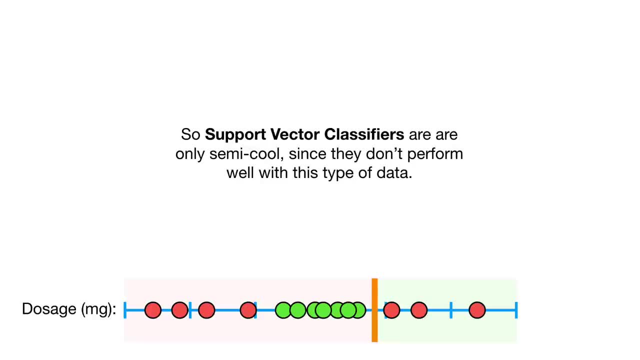 So support vector classifiers are only semi-quick, Since they don't perform well with this type of data, Since they don't perform well with this type of data, Since they don't perform well with this type of data, Can we do better than maximal margin classifiers and support vector classifiers? 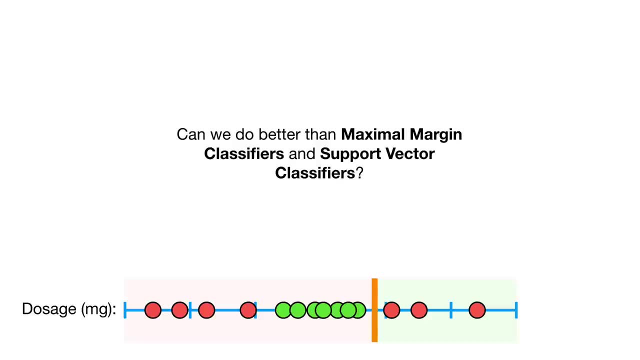 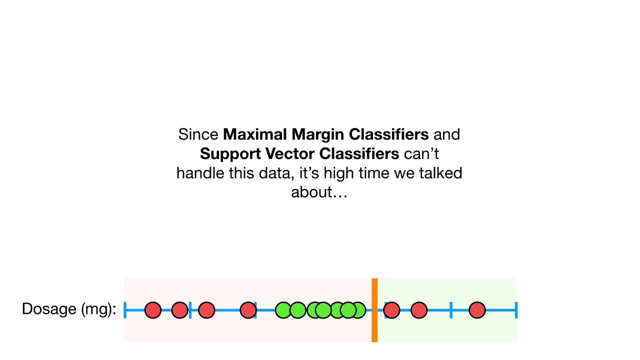 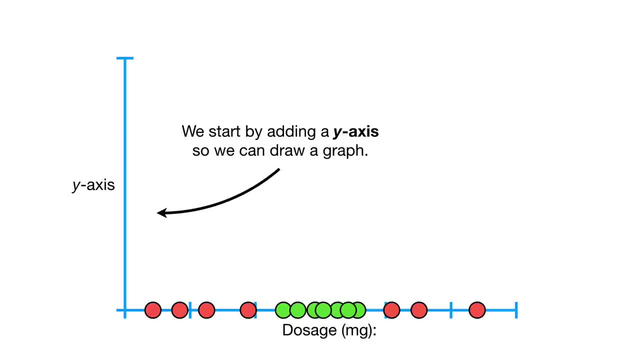 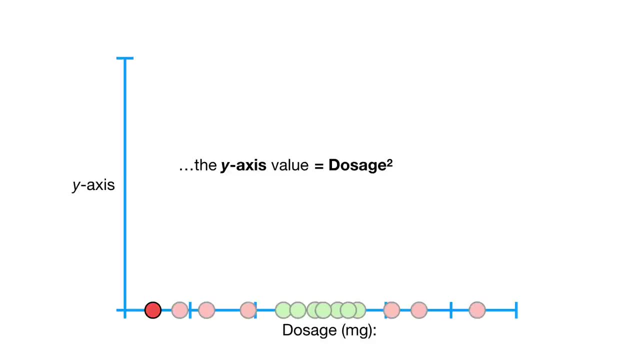 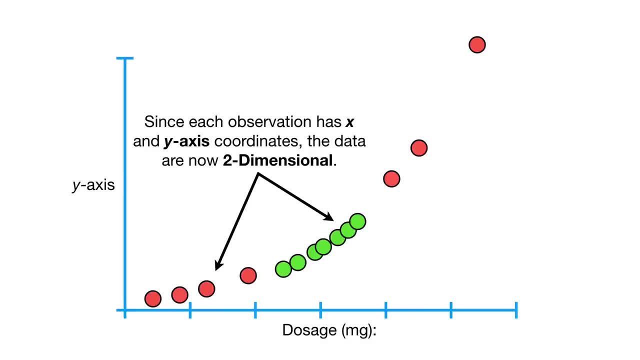 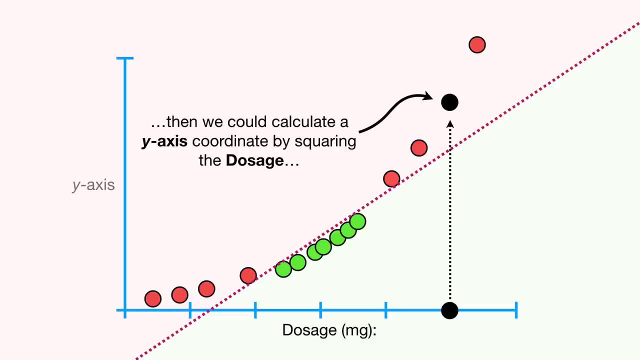 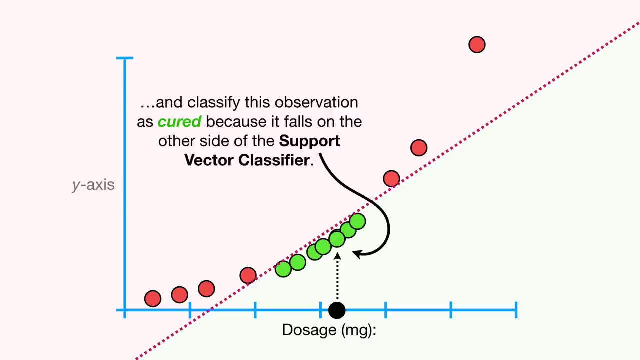 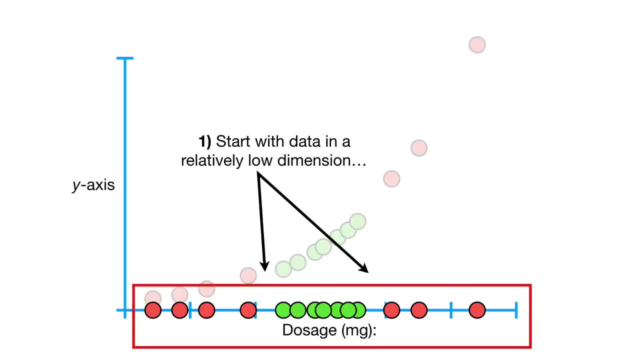 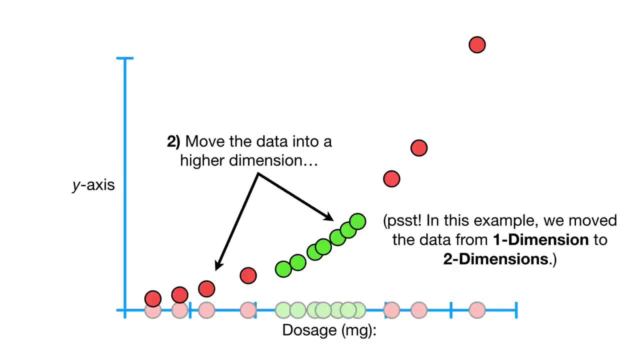 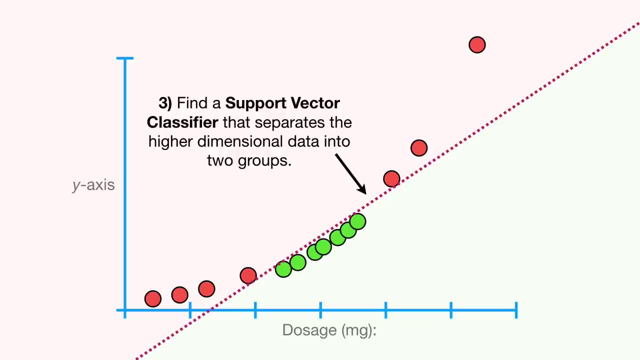 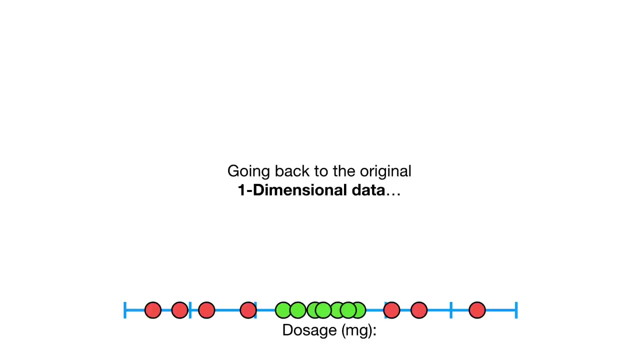 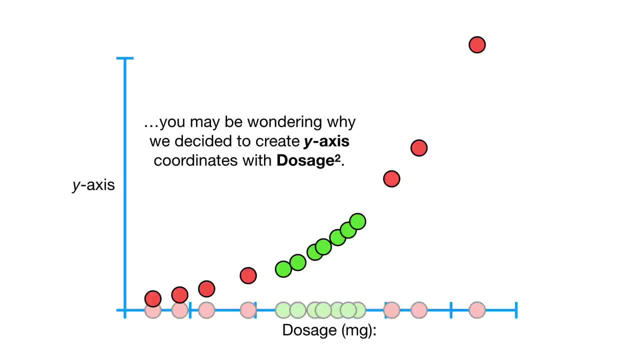 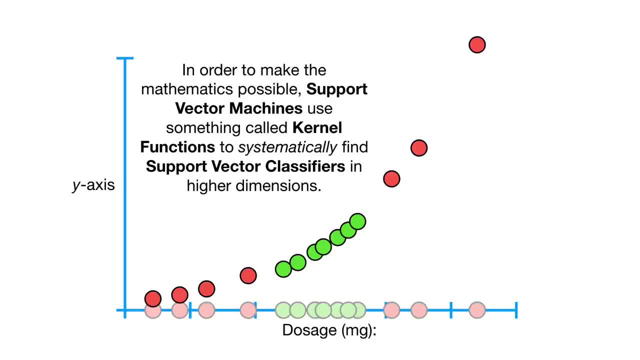 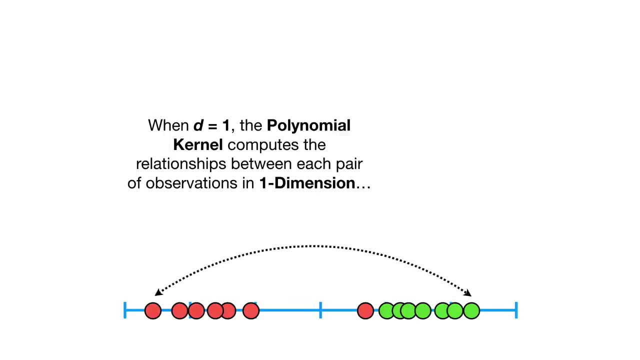 Yes, Thanks, Thank you, Thanks for your time. Any other question: polynomial kernel which has a parameter d, which stands for the degree of the polynomial When d equals 1, the polynomial kernel computes the relationships between each pair of observations in one dimension. 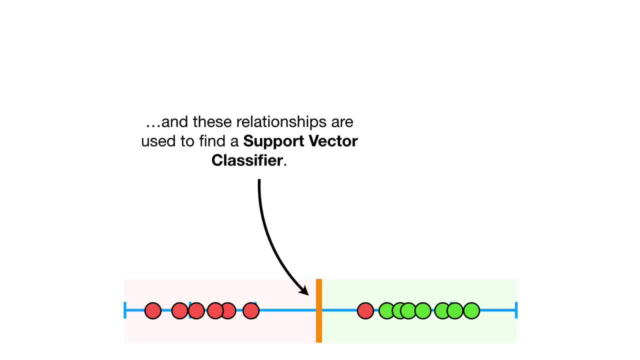 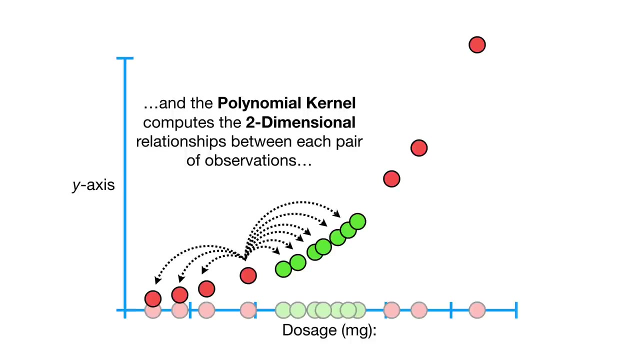 And these relationships are used to find a support vector classifier. When d equals 2, we get a second dimension based on dosages squared and the polynomial kernel computes the two-dimensional relationships between each pair of observations And those relationships are used to find. 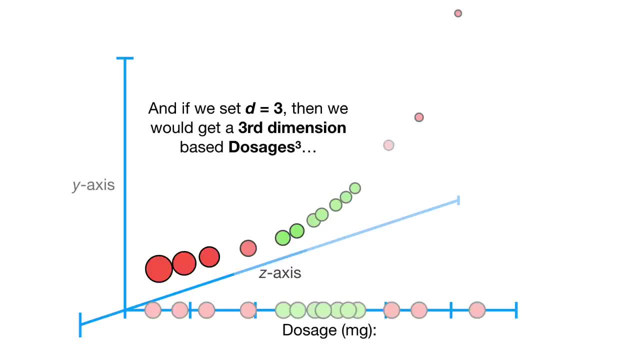 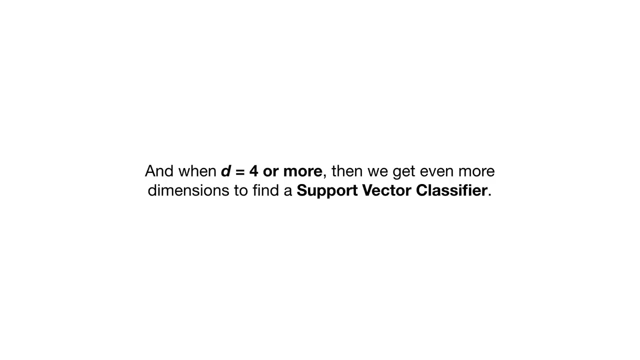 a support vector classifier. And when we set d equal 3, then we would get a third dimension based on dosages, cubed, and the polynomial kernel computes the three-dimensional relationships, the three-dimensional relationships between each pair of observations, And those relationships are used to find a support vector classifier. 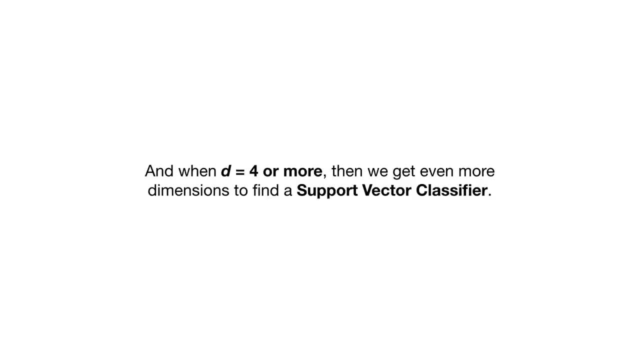 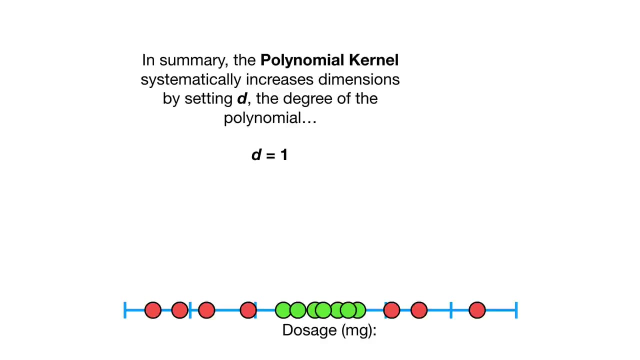 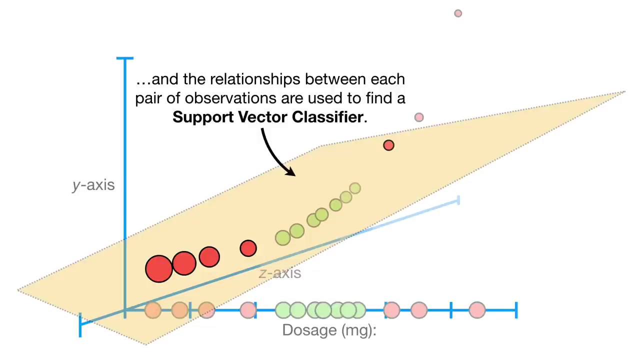 And when d equals 4 or more, then we get even more dimensions to find a support vector classifier. In summary, the polynomial kernel systematically increases dimensions by setting d, the degree of the polynomial And the relationships between each pair of observations are used to find a support vector. 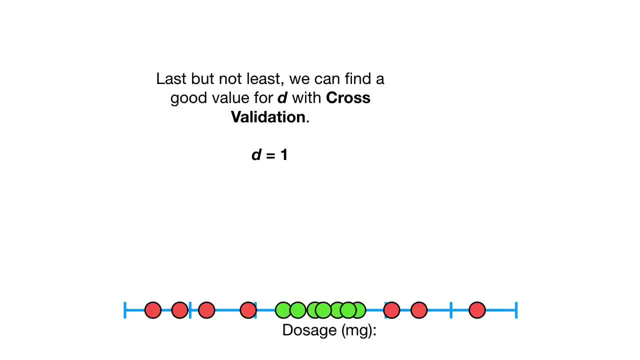 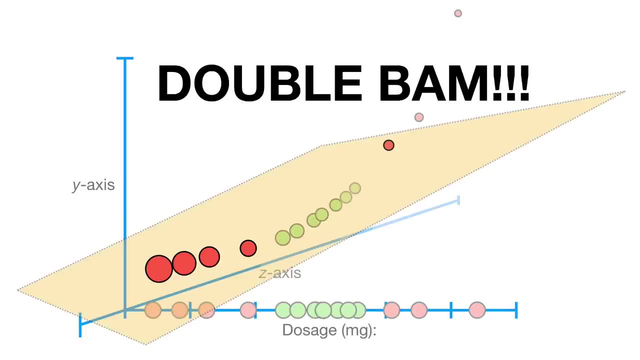 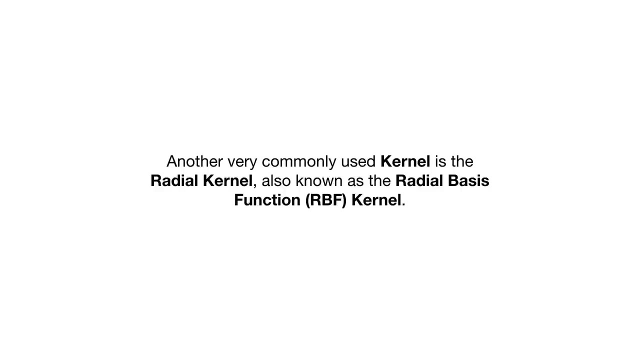 classifier. Last but not least, we can find a good value for d with cross-validation Double bam. Another very commonly used kernel is the radial kernel, also known as the radial basis function kernel. Unfortunately, Unfortunately, the radial kernel finds support vector classifiers in infinite dimensions. 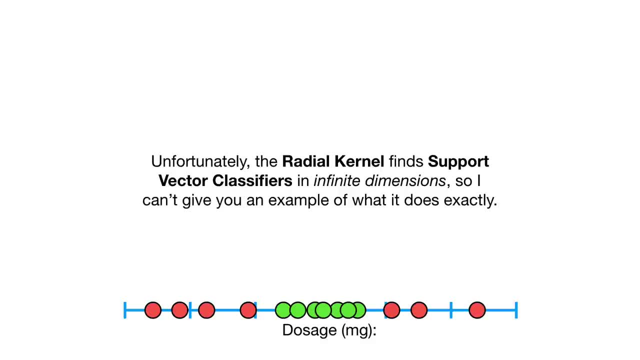 so I can't give you an example of what it does exactly. However, when using it on a new observation like this, the radial kernel behaves like a weighted nearest neighbor model. In other words, the closest observations, aka the nearest neighbors, have a lot of influence. 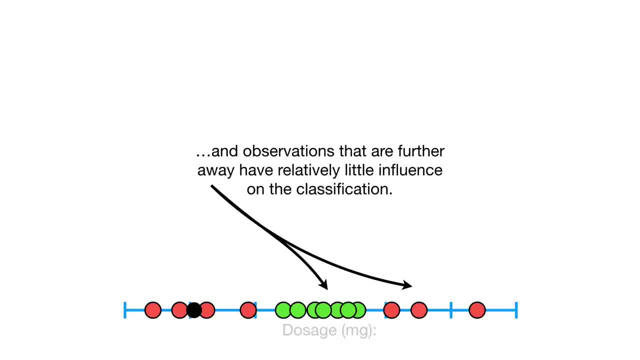 on how we classify the new observation. So what is the closest neighbor model? Well, the radius of the new observation is the radius of the new observation, And observations that are further away have relatively little influence on the classification. So, since these observations are the closest to the new observation, the radial kernel- 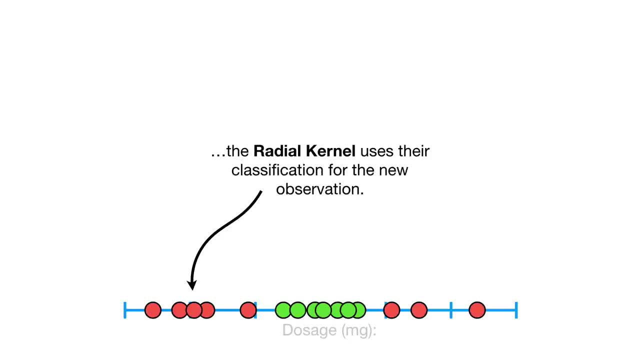 uses their classification for the new observation Bam. Now, for the sake of completeness, let me mention one last detail about kernels. The radial kernel is a function of the radial basis function. The radial kernel is a function of the radial basis function. 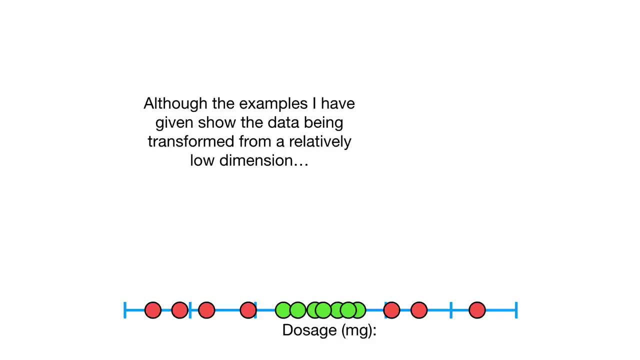 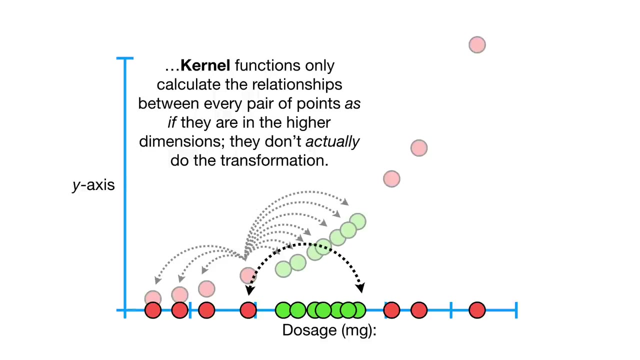 Although the examples I have given show the data being transformed from a relatively low dimension to a relatively high dimension, kernel functions only calculate the relationships between every pair of points as if they are in the higher dimensions. They don't actually do the transformation, This trick calculating the high dimensional relationships without actually transforming. 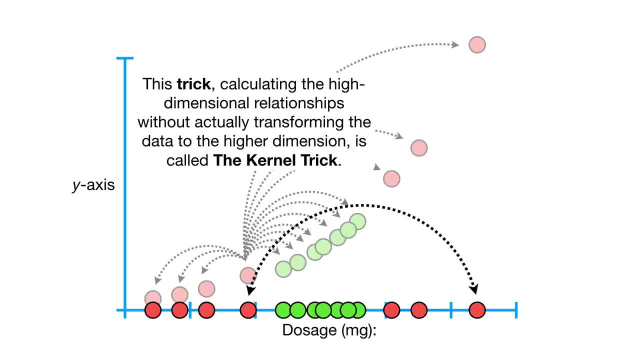 the data to the higher dimensions is a problem. So let's get back to our problem. higher dimension is called the kernel trick. The kernel trick reduces the amount of computation required for support vector machines by avoiding the math that transforms the data from low to high dimensions, And it makes